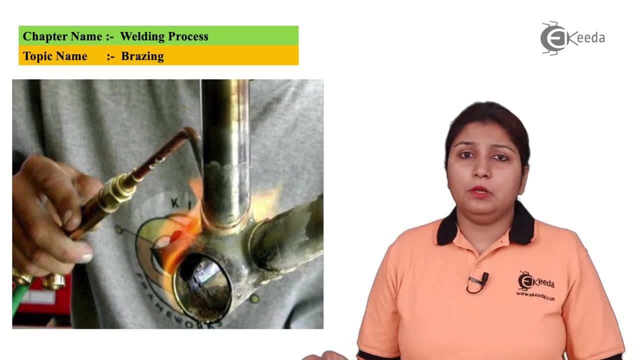 So in this diagram you can see there is an object, a pipe shaped object. nearly brazing are generally carried out at a pipe shaped object. A brazing gun is used. heat is eliminated from the brazing gun in the form of gas. 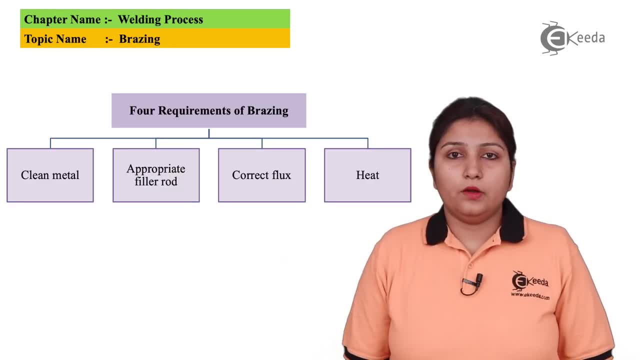 and brazing is done. So these are the four things which are required. Firstly, you need heat in the form of gas. Then you need a filler element. You also need flux. So these are some basic elements which are required while doing brazing. 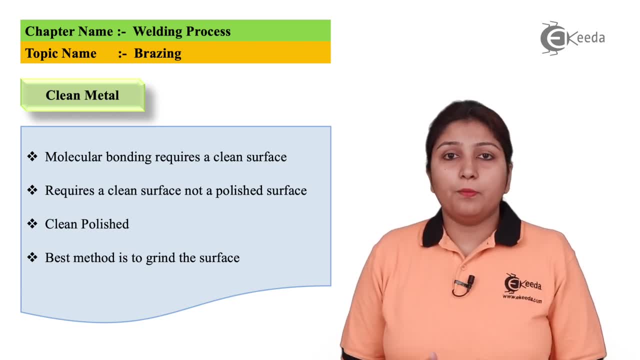 So a very essential factor which is required for brazing any of the object is clean and polished surface. The surface which is to be brazed, whether it would be a pipe, it would be a normal plain surface, any surface, it should be clean. 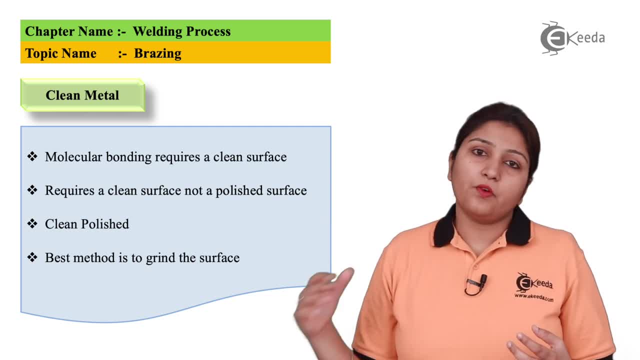 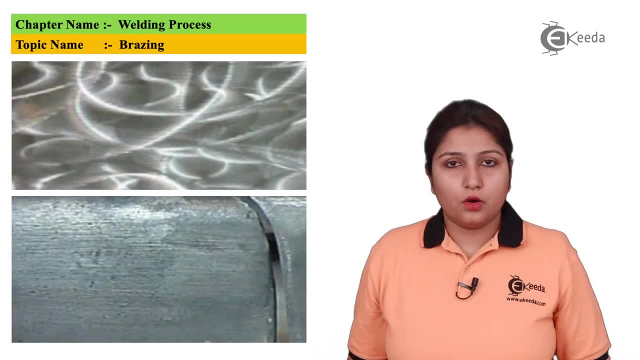 as well as polished. You can see the two diagrams. the first diagram is of a clean surface and the second diagram is of a polished surface. In this diagram you can see there is a filler rod. Generally for brazing you use a filler rod which is flux coated. 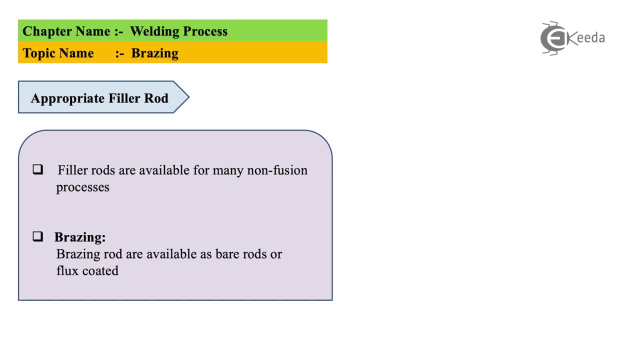 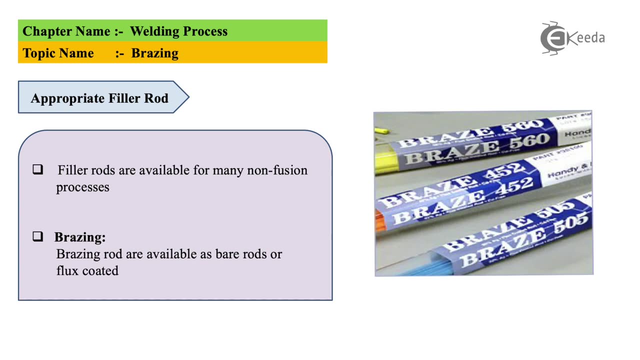 The flux is already coated on the filler rod So it can be easily used. Also, your rod should also be clean. In brazing, cleanliness is a major factor for doing your exact joining process. So this is flux. It is available in all the three forms, like paste, powder or liquid. 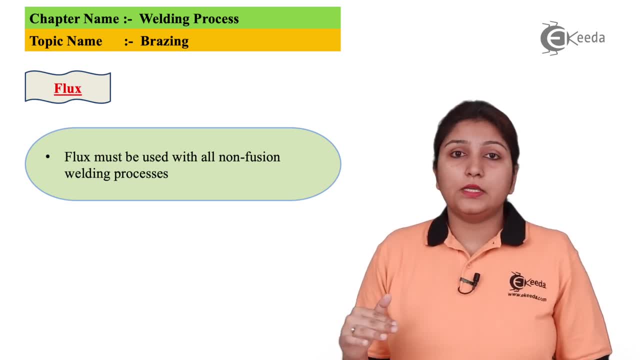 So, according to the requirement, the flux can be used in your brazing process. So it can be coated, it can be sprayed, whatever form you use it exactly Now? the next factor is heat. Sufficient heat is required for brazing. 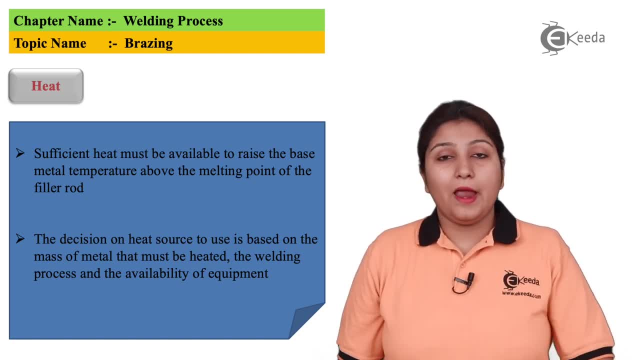 If heat is less, your brazing cannot be done properly And the amount of heat required, like the decision of giving the heat supply, depends on your metal, Like if, say, the metal is thick, heating is more. If the metal is thin, heating is less. 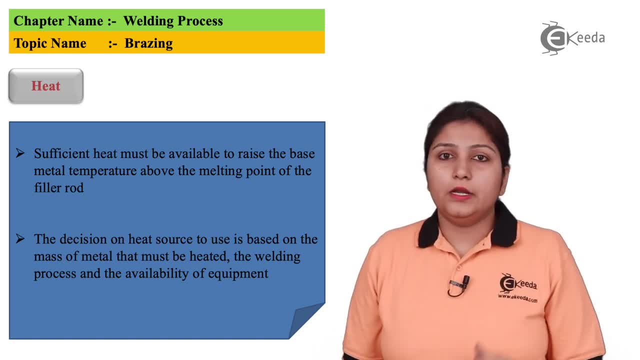 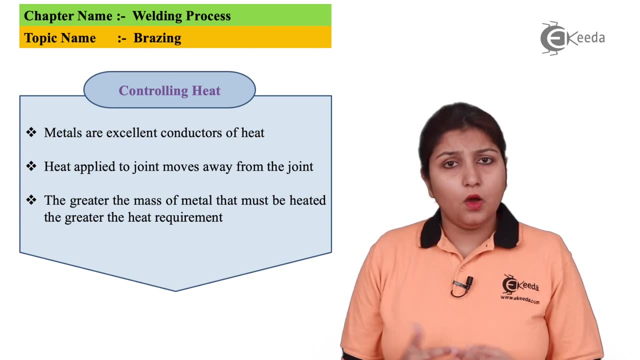 So depending on your metal size or your metal thickness, heating can be given. So, according to brazing rules, heating depends on the material. Also, controlled heating is required. So if excess heating is provided, the joint may fail or it can become dirty. 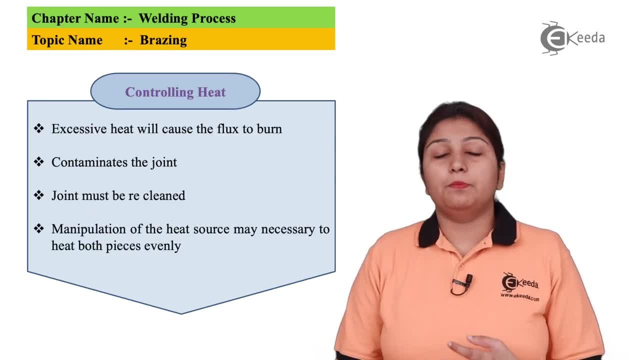 So for keeping the flux in proper position, keeping the metal properly welded, heating is an important factor. So controlled heating is required so that you can use your flux properly, you can join the metal properly. Also, the joint may not break before it is supposed to break. 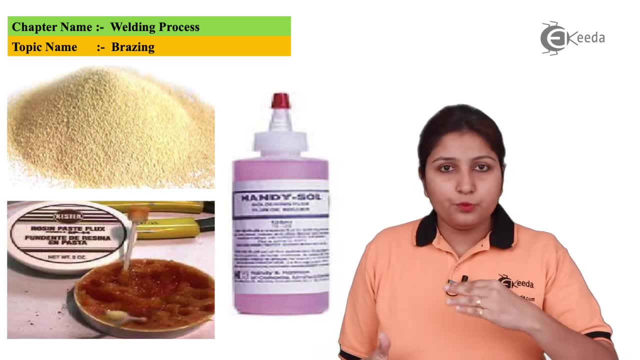 So, in brief, I will tell you all the brazing processes, Like the steps which are following, for brazing is: firstly, you have to take your material to be brazed- two or three materials together, as we have seen in our diagram. 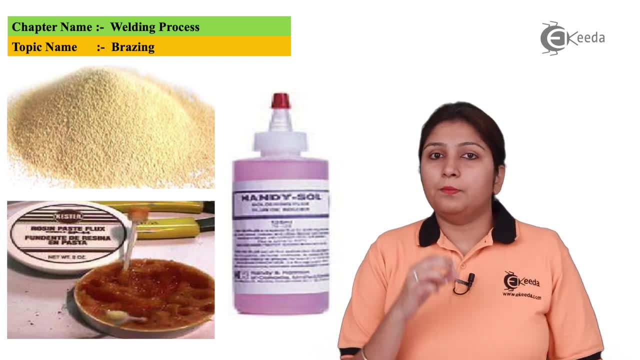 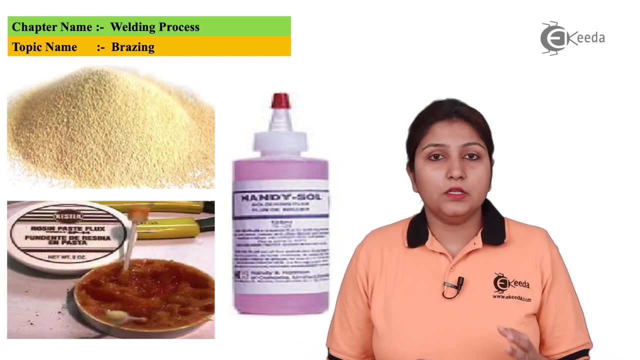 Then your brazing gun is used. It has some heat source, Heat is coming, But before that your surface to be brazed has to be cleaned. So the brazing surface gives proper heat to your surface to be brazed. 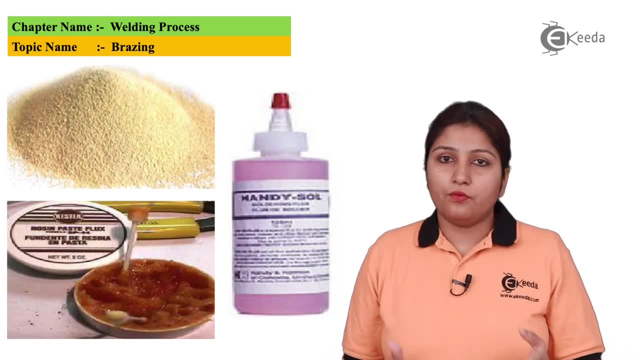 Then what happens is another filler element or your filler metal is added, which is flux coated, or at times, additional flux can be added in the form of powder, liquid paste, etc. So in this way your exact brazing action takes place. 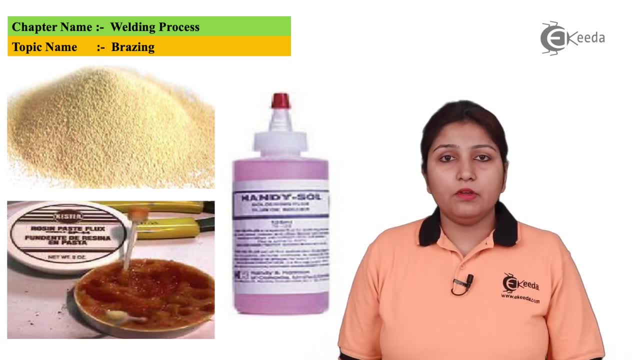 So after the brazing we are leaving the metal to get solidified. The braze weld exactly should be solidified and the whole process is completed. So in this diagram you can see there are two parts. One is your joining process. 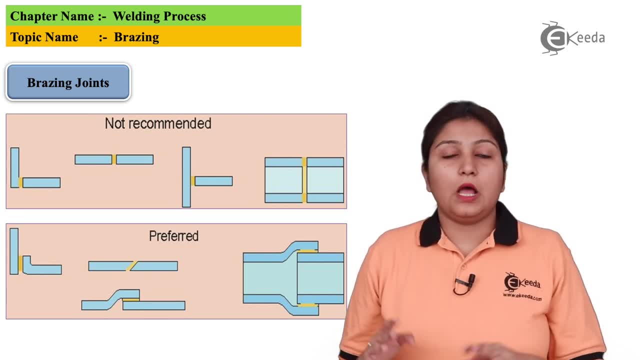 Second is exactly preferred joining process, How brazing should be done So you can see: if a lap joint is used, the surfaces should be in a bent way. If a butt joint is used, the surface should be in an angular way. 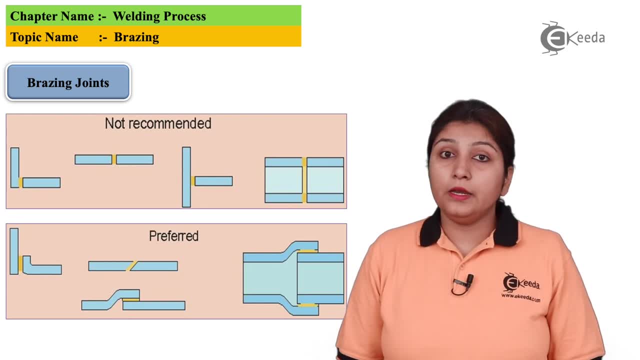 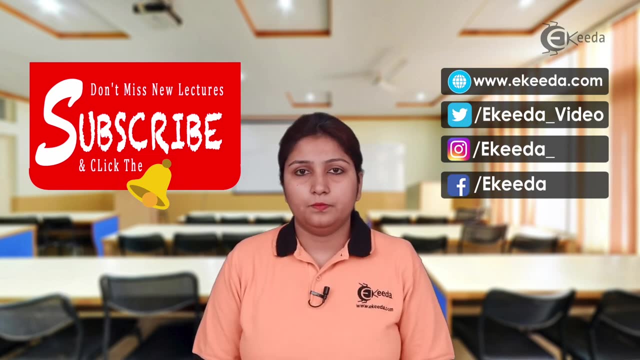 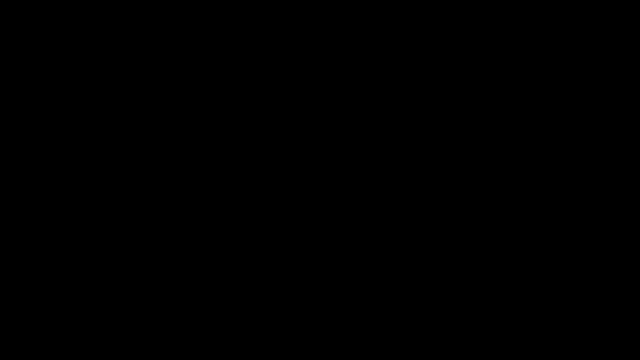 In a similar way. the other two joints are explained in brazing process. Thank you for watching this video. Stay tuned with eKIDA and do subscribe our channel, eKIDA, wwweKIDAcom.